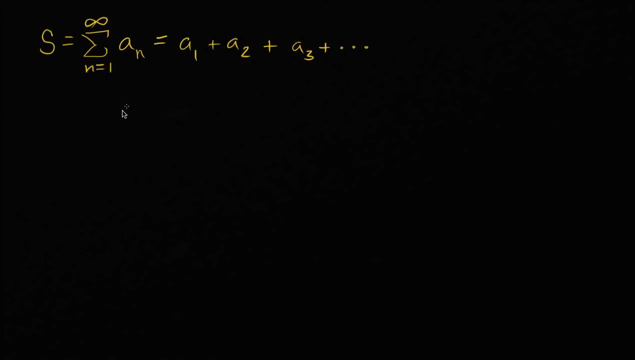 This right over here is an infinite series, But we could define a partial sum. so if we say S sub six, this notation says okay, if S is an infinite series, S sub six is the partial sum of the first six terms. 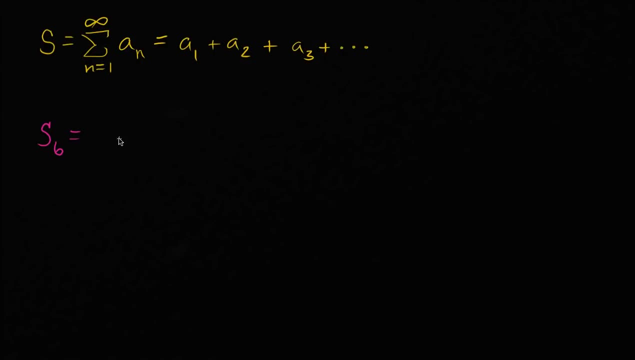 So in this case, this is going to be- we're not gonna just keep going on forever. this is going to be a sub one plus a sub two plus a sub three Plus a sub four plus a sub five plus a sub six. 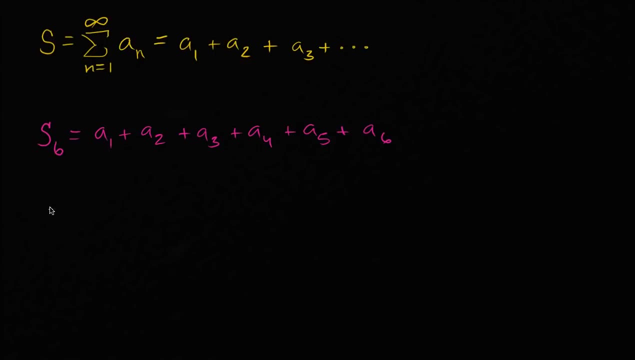 And I could make this a little bit more tangible if you like. So let's say that S, the infinite series, S is equal to the sum from n equals one to infinity of one over n squared. In this case it would be: let's see: 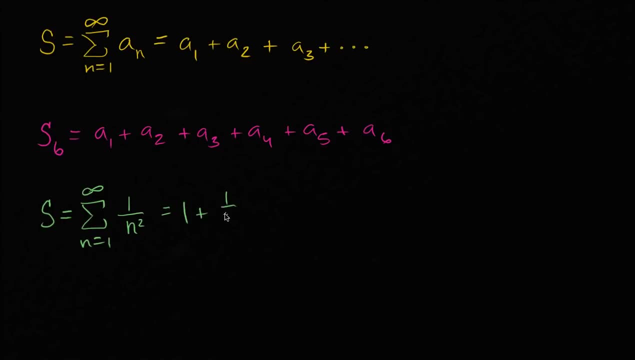 one over one squared, plus one over two squared, plus one over three squared, And we would just keep going on and on and on forever. But what would S sub? actually? let me do that same color. What would S? I said I would change color and I didn't. 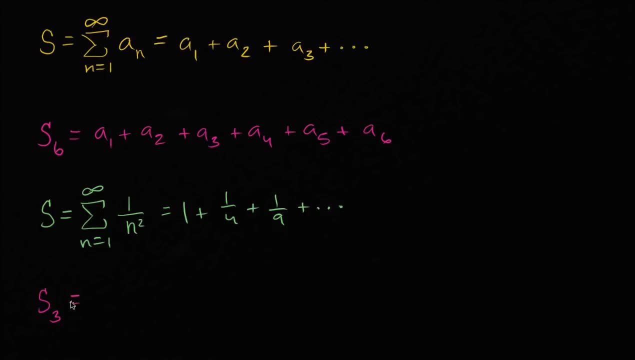 What would S sub three be equal to The partial sum of the first three terms, And I encourage you to pause the video and try to work through it on your own. Well, it's just going to be. this is going to be the first term. 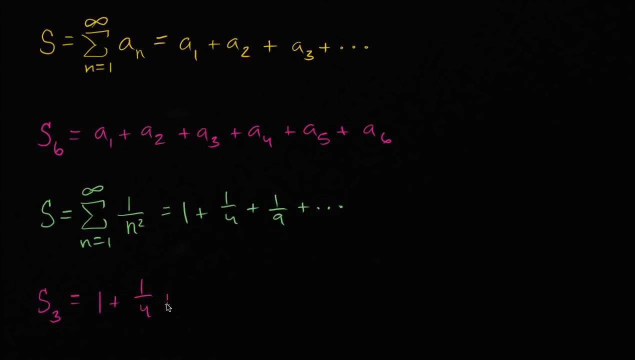 One plus the second term. one fourth plus the third term, one ninth. It's going to be the sum of the first three terms And we could figure that out. Let's see if we have a common denominator here. It's going to be 36.. 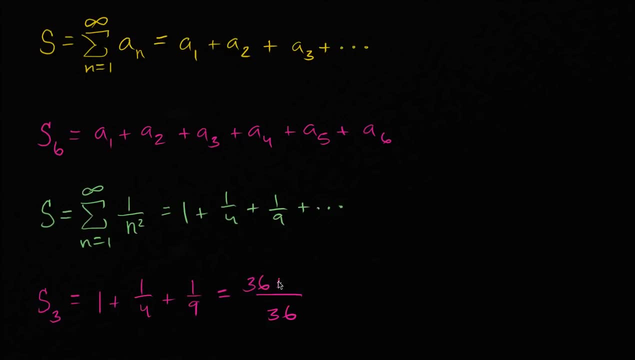 It's going to be 36 thirty-sixths plus nine thirty-sixths plus four thirty-sixths, So this is going to be 49 over 36.. 49,, 49 over 36.. So the whole point of this, the whole point of this video, is just to appreciate. 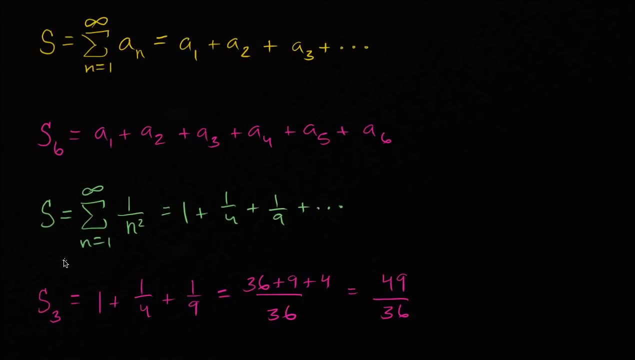 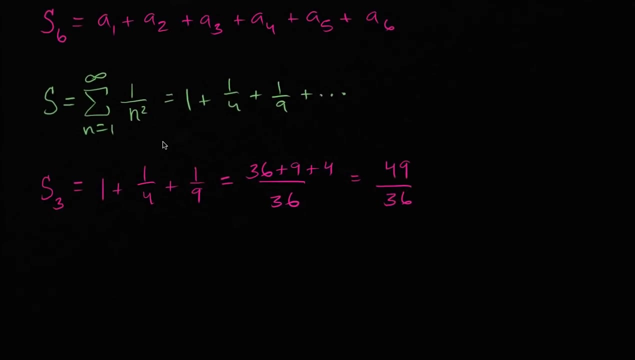 this idea of a partial sum, And what we'll see is that you can actually express what a partial sum might be algebraically. So for example, for example, let's give ourselves a little bit more real estate here. Let's say, let's go back to just saying: 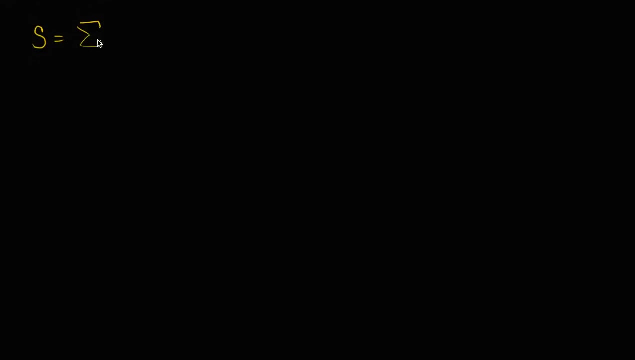 we have an infinite series, S that is equal to the sum from N, equals one to infinity of A sub N. And let's say we know that the partial sum, the partial sum S sub N, so the sum of the first N terms of this, 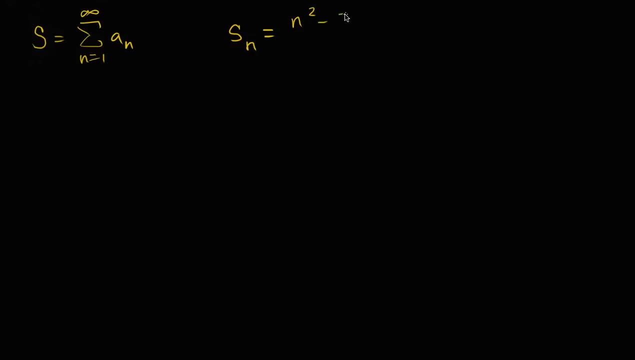 is equal to N squared minus three over over N to the third plus four. So just as a bit of a reminder of what this is saying: S sub N, S sub N is the same thing as A sub one plus A sub two plus you keep going all the way to A sub N. 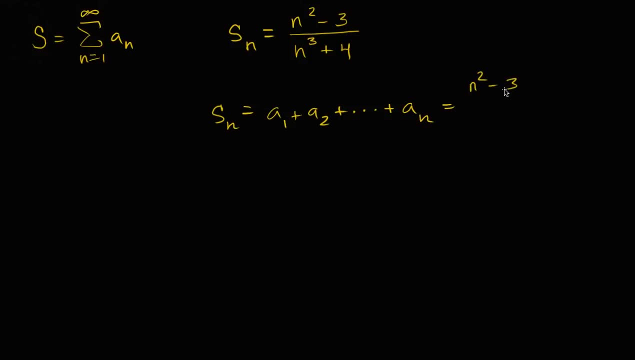 And that's going to be equal to this business: N squared minus three over N to the third plus four. Now, given that if someone were to walk up to you on the street and said, okay, now that you know the notation for a partial sum, 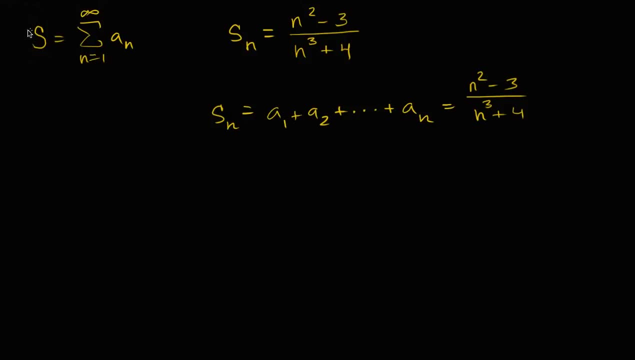 I have a little question to ask of you. If this is, if S is the infinite series- and I'm writing it in very general terms right over here- So S is the infinite series. from N equals one to infinity of A sub N. 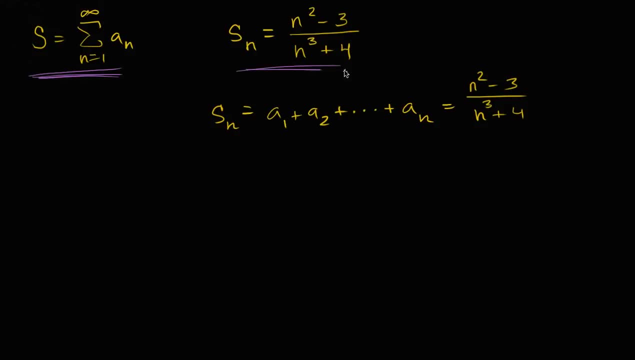 The partial sum S sub N is defined this way. So someone, they tell you these two things And then they say, find, find what the sum from N equals one to six- of A sub N is. And I encourage you to pause the video. 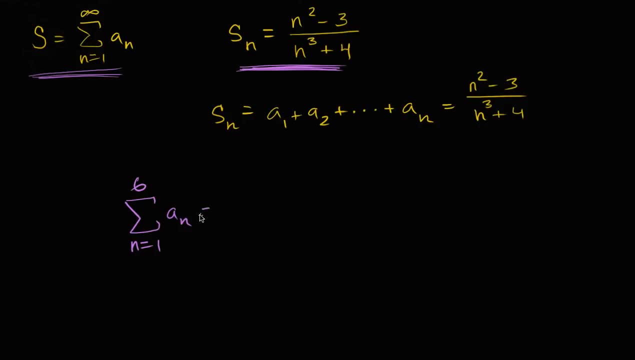 and try to figure it out. Well, this is just going to be. this is going to be A sub one plus A sub two, plus A sub three plus A sub four, and when I say sub, Let's say sub, that just means subscript. 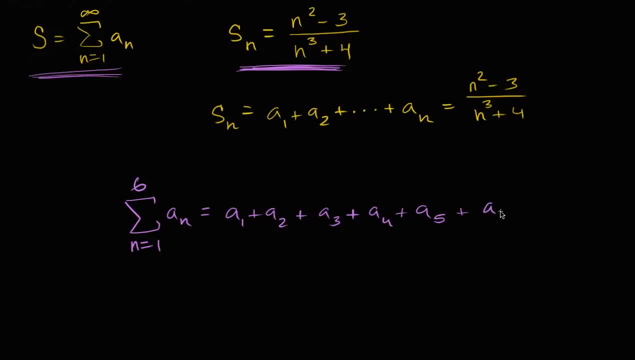 plus a sub five plus a sub six. Well, that's just the same thing as the partial sum. This is just the same thing as the partial sum of the first six terms for our infinite series. This is going to be the partial sum s sub six. 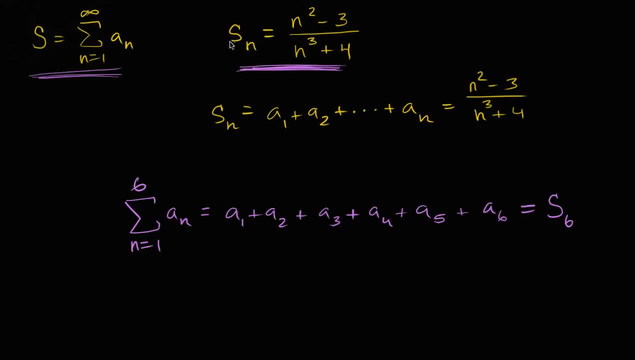 And we know how to algebraically evaluate what s sub six is, We can apply this formula that we were given s sub six is equal to well. everywhere we see an n, we replace with a six. It's going to be six squared minus three.